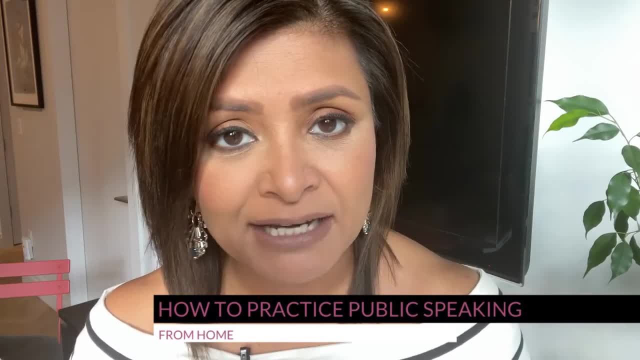 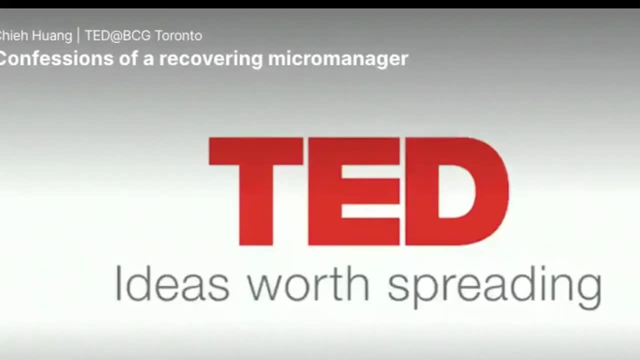 your paper the whole time. Let's build that awareness muscle and make note of it All right. Tip number three is to watch other great talks. I love the Ted talk that my friend Che Huang gave. He's the CEO of Boxcom. 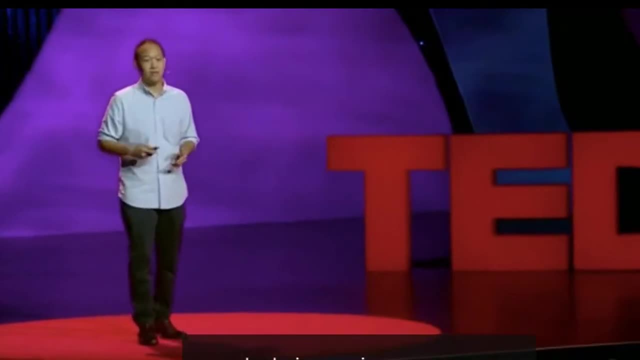 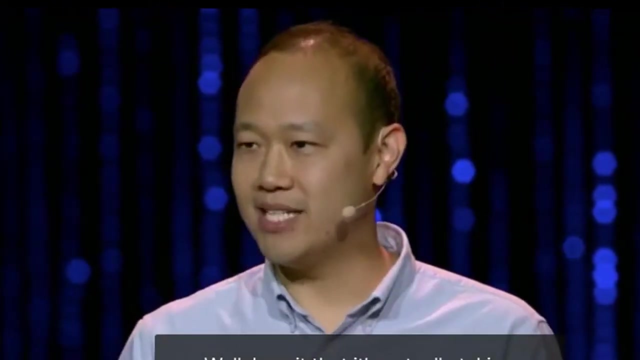 This is a company whose valuation is well over $600 million, And he could have talked about a number of things as it relates to building a very successful wholesale products business, But he chose to talk about one thing and one thing only. He kept the message super simple. 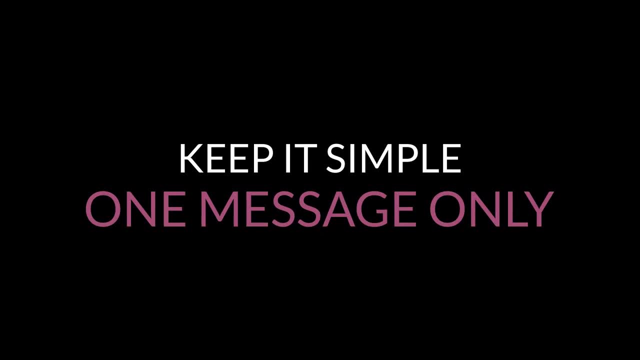 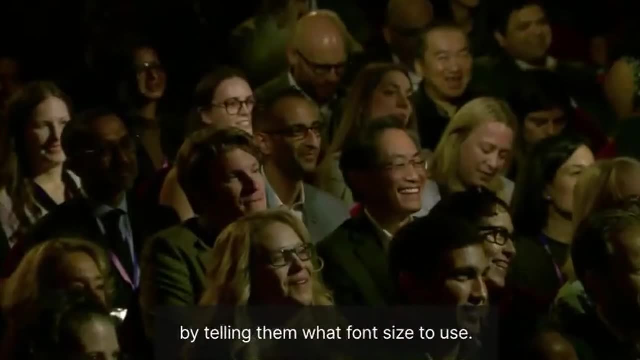 which is the art of managing people. That is the only thing he talked about, So content is one piece of it, which is why you watch other great talks, but also watch their mannerisms. What are they doing with their eye contact? What are they doing with their hands? 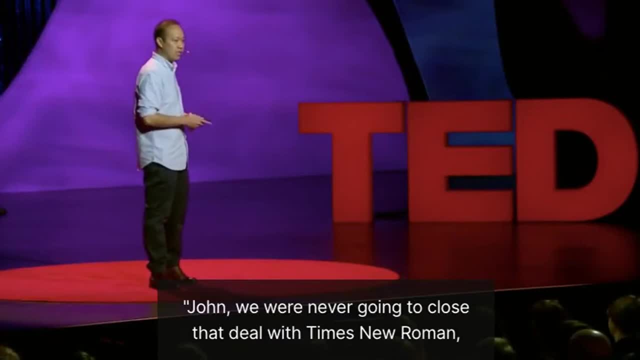 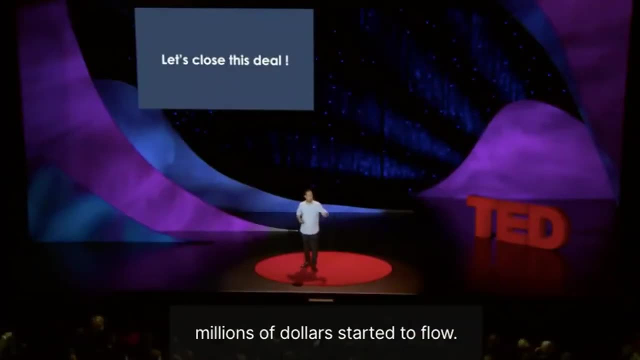 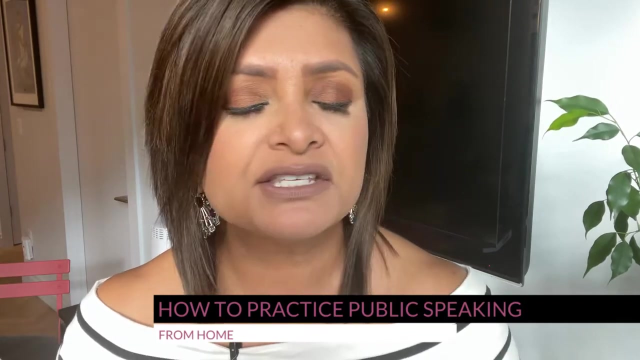 Are they walking, Are they standing still, Are they leaning forward? Write down five things that you see other people that are doing really, really well, and see if you can integrate one of those things into the way that you present. Two other bonus talks that I really love: Steve Jobs commencement speech at Stanford in 2005.. Look it up on YouTube. 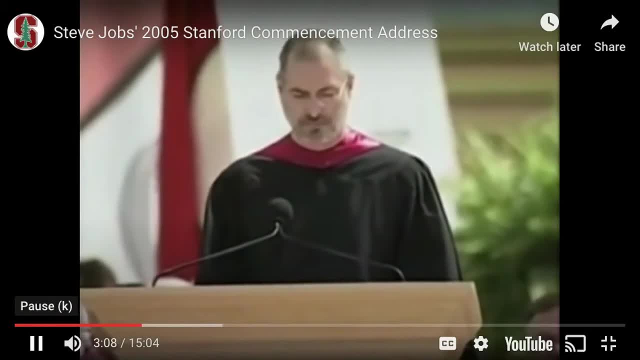 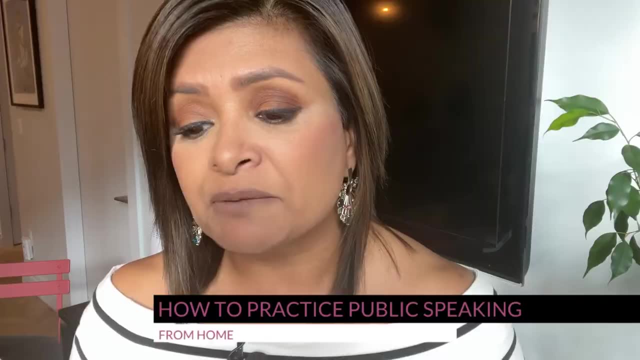 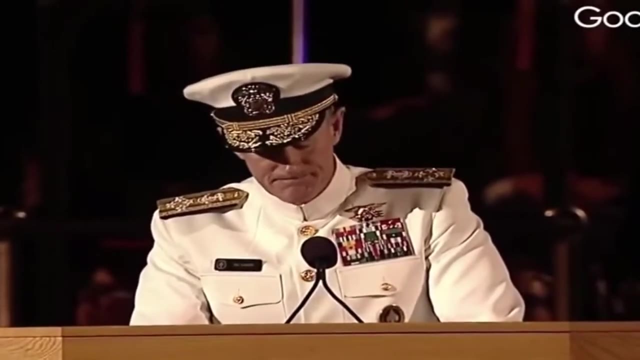 It's a great, great talk. Gives me chills every time I hear it, But this is a man who is so confident in his delivery. The other talk that I really love was by Admiral William McRaven. He is a former Navy admiral and he wrote a book. He also gave a Ted talk called Make Your Bed. 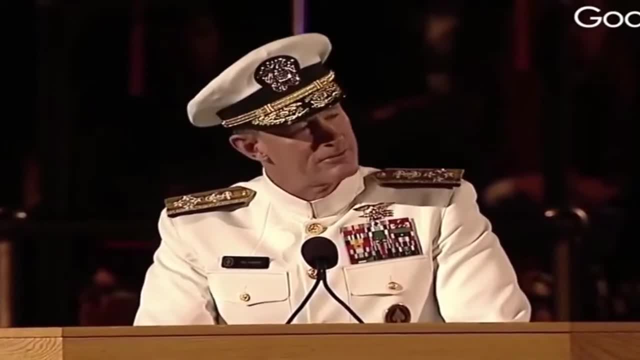 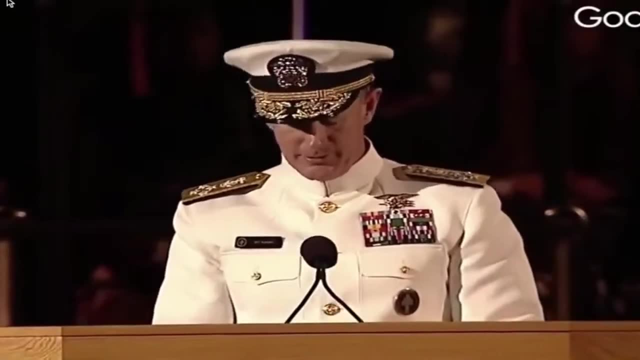 With the ethos that you should make your bed first thing in the morning because there's a ripple effect on how the rest of your day is going to go. It gives you a sense of accomplishment. So number one, just to recap, is to make your bed first thing in the morning. 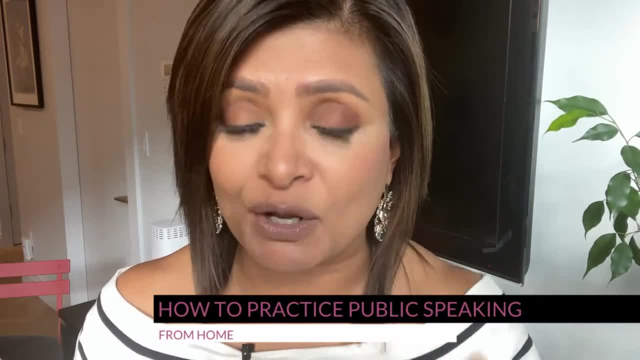 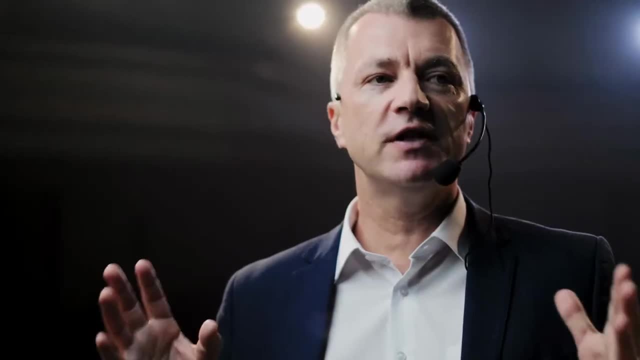 Number two is to record yourself daily. Number two is to play it back, once with the volume up, once with the volume down, to build self-awareness around what it is that you're doing. And then number three is to watch other great talks to see what other great people are doing. 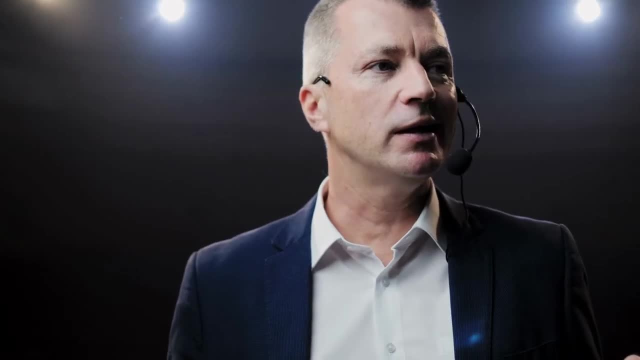 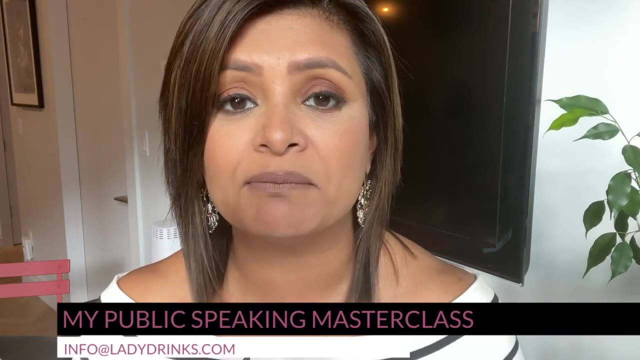 to give really impactful speeches. Okay, I'm in the middle of teaching a public speaking masterclass. This second cohort of seven power women is already underway, but I welcome you to join me for the next cohort of seven power women. My masterclass kicks back up.